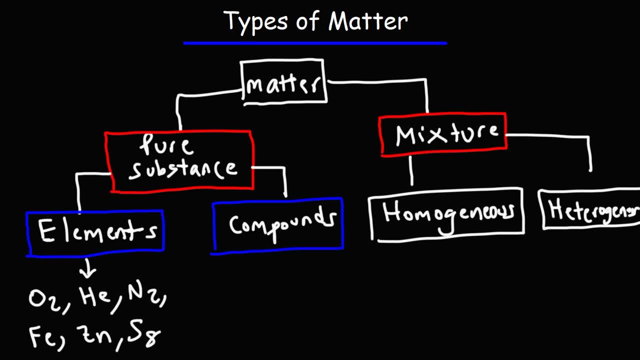 sulfur. These are all pure substances and each of these substances they're composed of only one kind of element. So that's an example of a pure substance. Now, compounds also are part of pure substances. So water is a compound, but it's also a pure substance. Now, what makes it a compound is that water is. 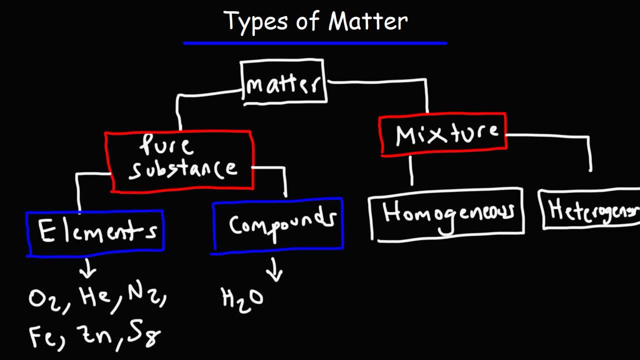 composed of two different elements. So any substance that is composed of two or more different kinds of elements are compounds. Sodium chloride is a compound. It's a pure substance, but it's made of two different elements. Ethanol is a compound. It's made up of the elements carbon hydrogen and oxygen. 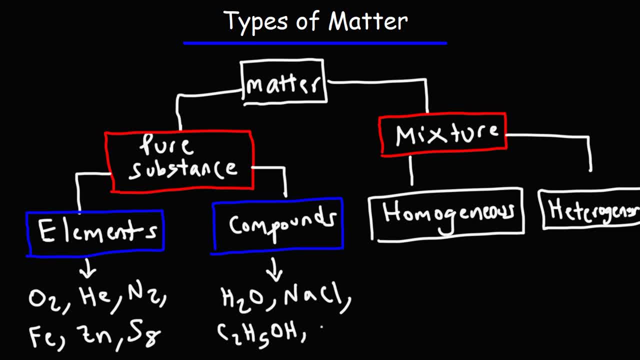 but it's only one kind of pure substance: Carbon dioxide. you know that's a pure substance. By the way, for those of you who want more example problems on pure substances and mixtures, check out the links in the description section below. I'm going to post some more video content on this. 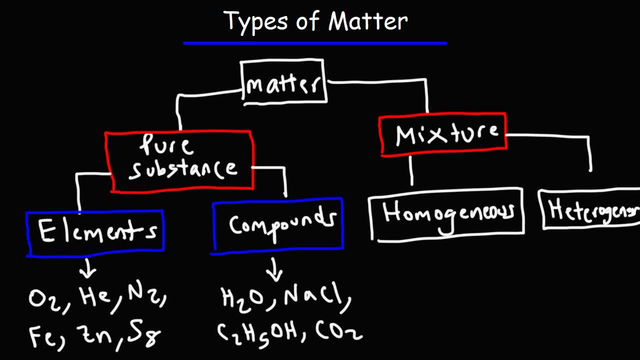 topic in addition to homogeneous and heterogeneous mixtures. So feel free to take a look at that when you get a chance. Now, on the right side, we have two different kinds of mixtures Now. a homogeneous mixture is one where the composition is uniform, So salt and water. that is a homogeneous. 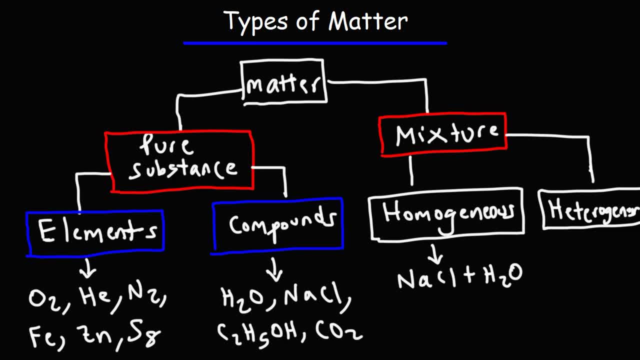 mixture. Remember. a mixture is basically two or more pure substances that are combined with each other. When you mix salt and water together, it's going to appear as one clear solution. The salt mixes uniformly with the water and that makes it a homogeneous mixture. 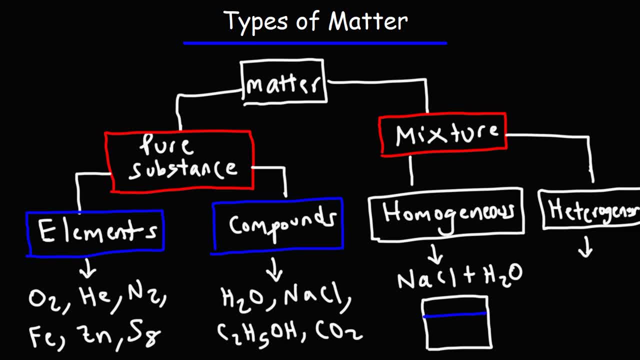 A heterogeneous mixture. you don't have that uniform composition. So oil and water would be a good example of a heterogeneous mixture. So when you mix oil and water, they actually don't mix. The oil, being less dense than water, is going to float on top. It has a lower density in water. So here is the oil.